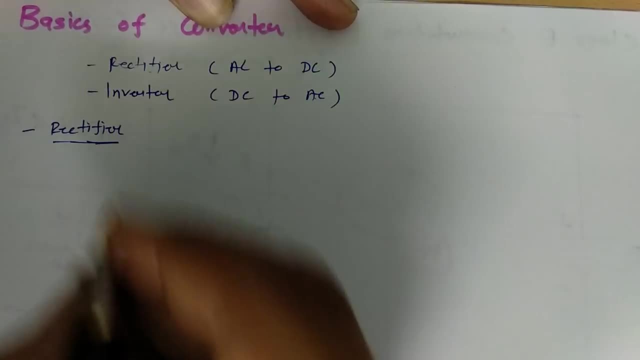 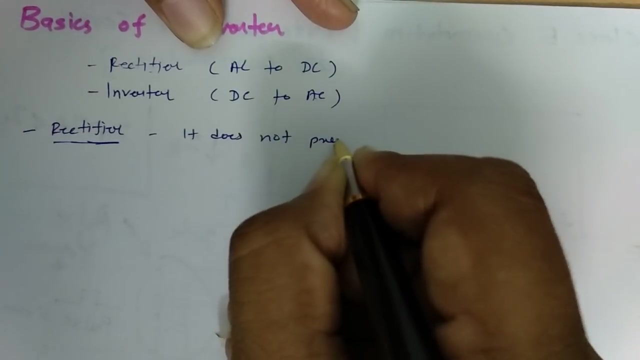 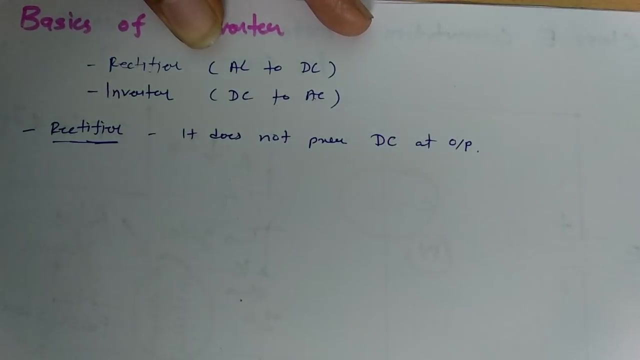 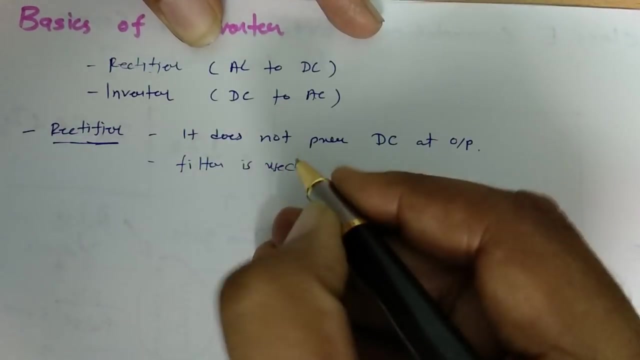 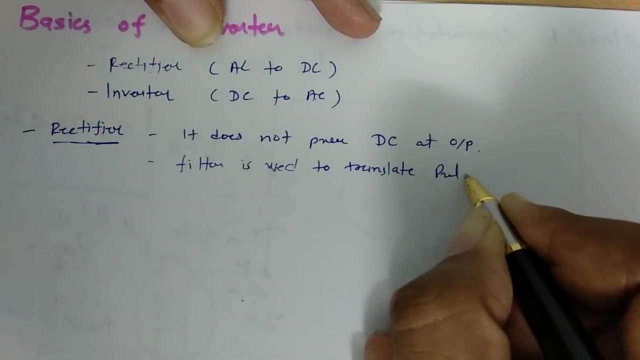 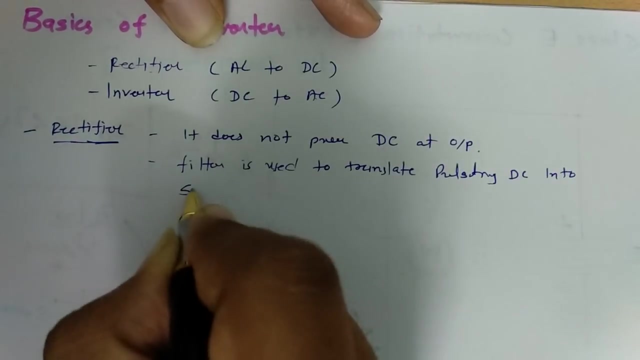 DC from AC. Then we use rectifier, So rectifier circuit. it does not give pure DC at output, But at the end, by connecting filter, we can translate pulsating DC into smooth DC. So filter is being used To translate pulsating DC into smooth DC. Now to understand that, I will give you one basic. 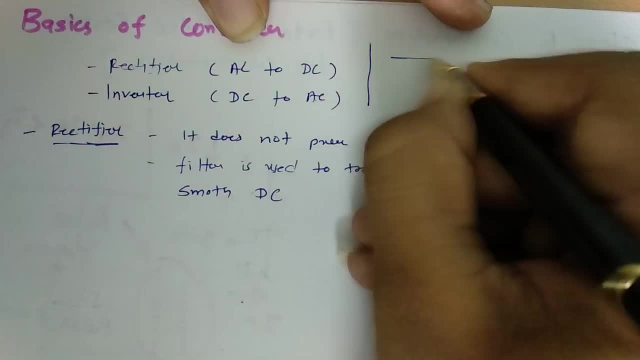 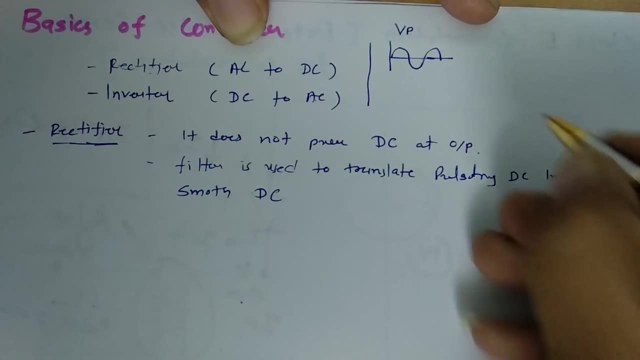 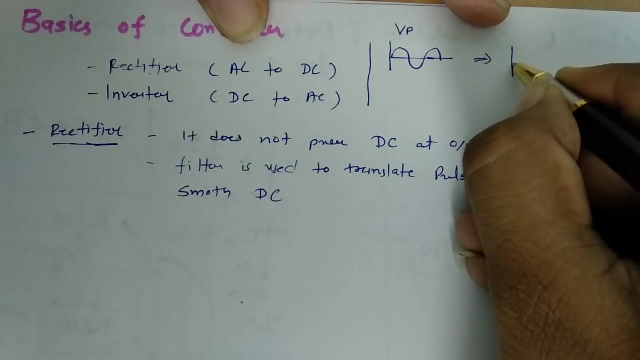 example Like: see, for example, if you have AC input, so this is what AC input that is there with us. So this is input. Now, by using rectifier circuit, we translate that into DC, but that is pulsating DC. So this: 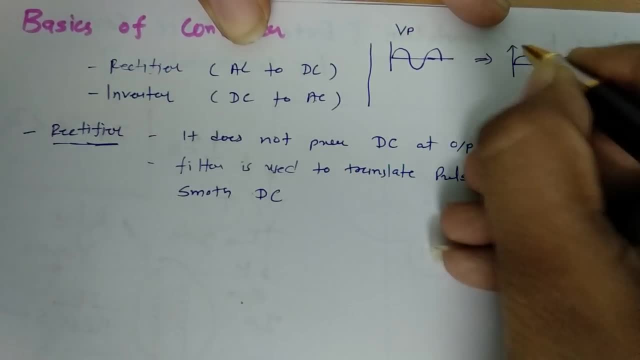 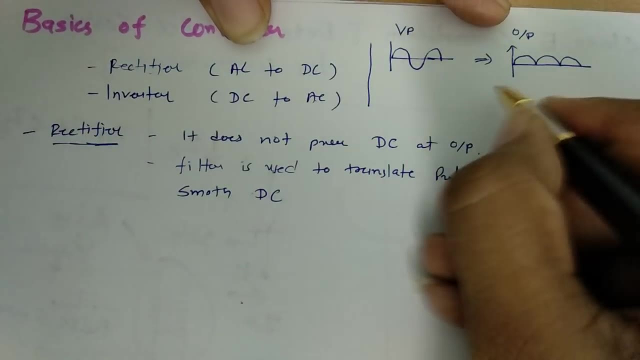 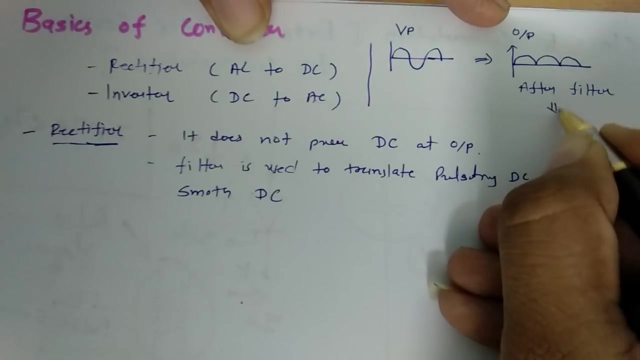 is what my output. This is full wave output of rectifier, but this is pulsating DC. Now by using filter, we can translate this in smooth DC DC. so after passing through filter, we will be having smooth DC like this, and by having 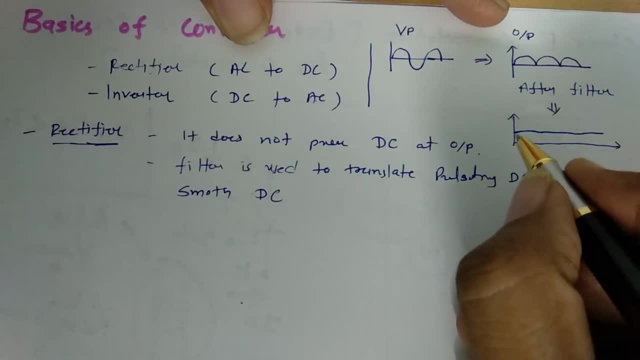 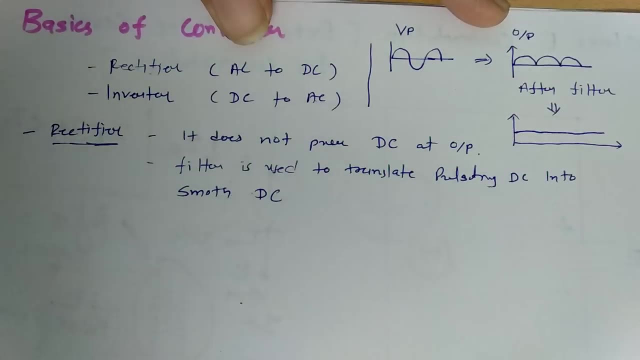 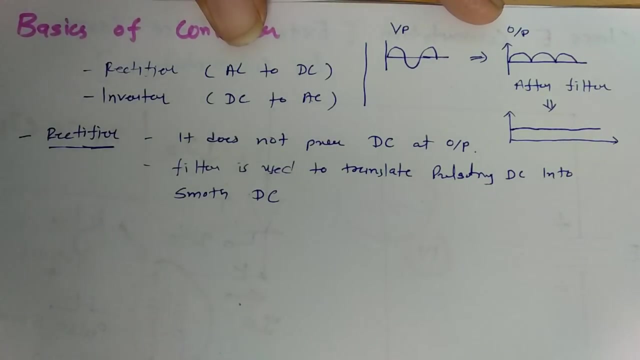 increase in order of filtration, we can increase its smoothness. so that depends on which type of filter that we are using and that one can understand it. in my preceding videos, where I have explained how we can have a filtration, I have explained the use of filter by using 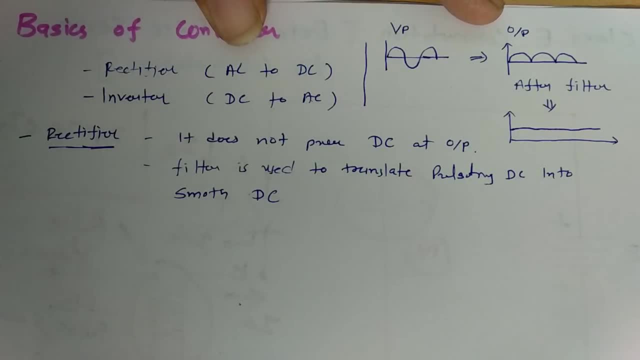 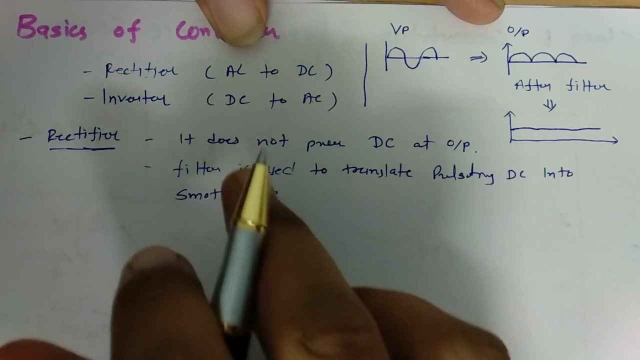 capacitor, by using inductor, by using pi filter. so that will give you clear idea about how we can have filtration to have smooth DC from pulsating DC. so, ultimately, rectifier that is translating AC signal into DC signal. initially it will be pulsating DC signal- and by using 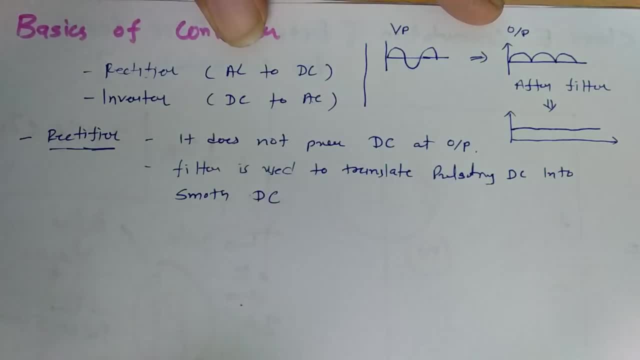 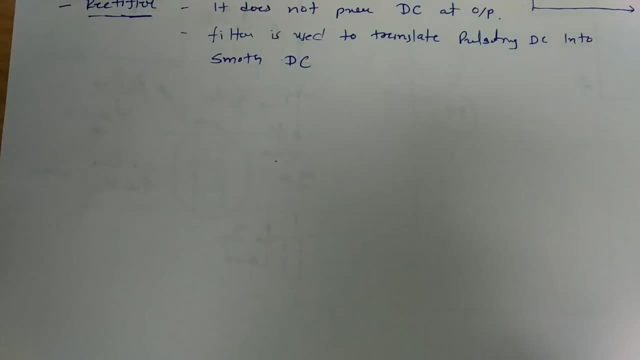 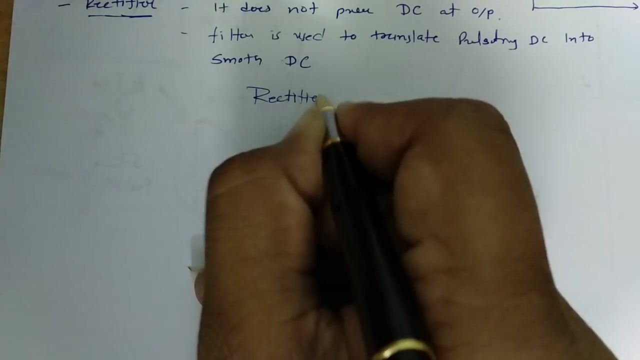 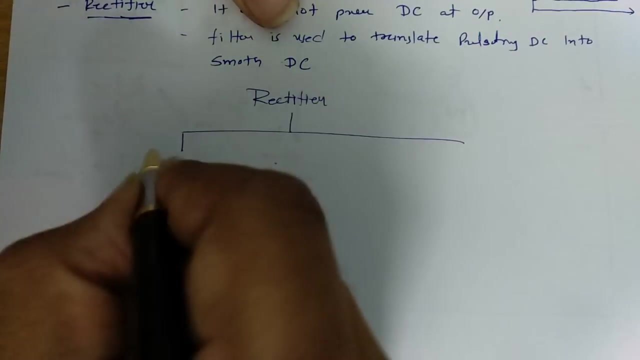 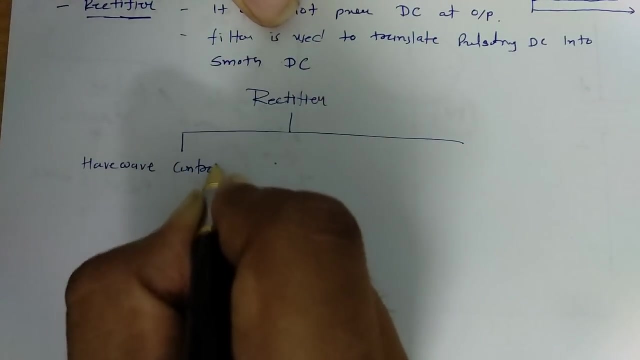 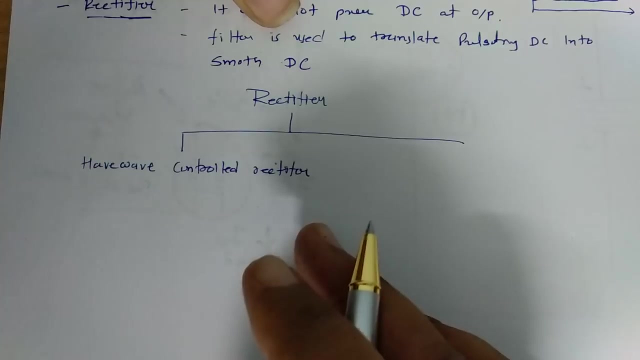 filter we can convert this pulsating DC into smooth DC. now first I will explain how many things that I will be explaining in rectifier portion. So in rectifier I will explain controlled rectifier. so I will explain half wave controlled rectifier. So here I will explain single phase half wave controlled rectifier. 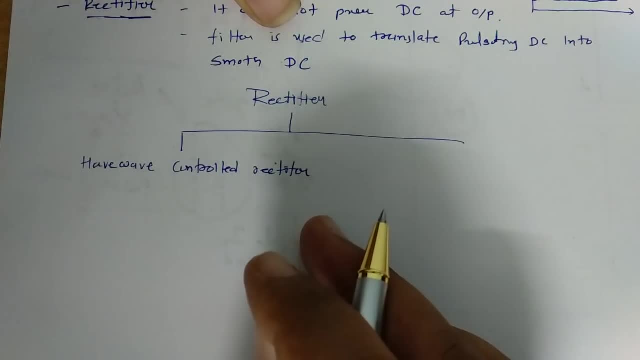 and in that I'll explain. if we have load which is resistive load, then what could be our output? then in case of inductive load, what could be our output? and there are few problems, as if we have connection of inductive load and to overcome that we can have a connection of freewheeling diode. 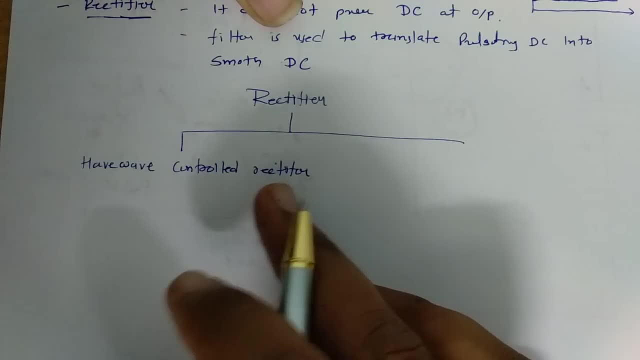 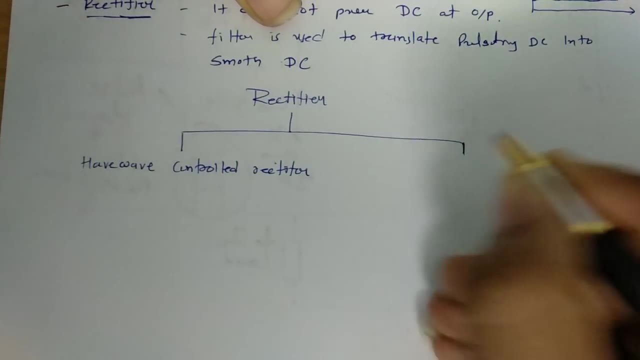 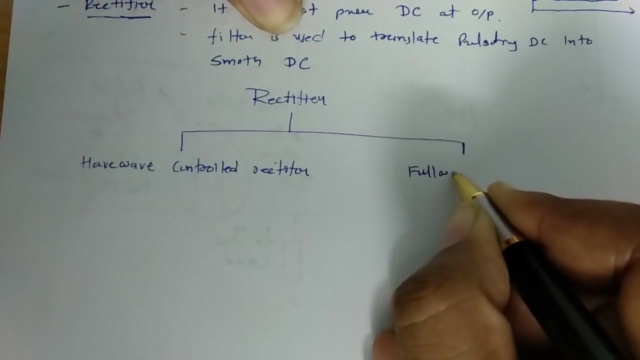 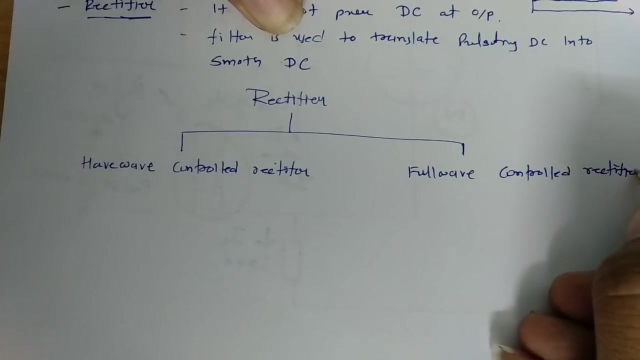 so what are the changes which will happen after connection of freewheeling diode? that is what I will be explaining in this and then second phase that I'll be explaining with full wave controlled rectifier. so where, in full wave controlled rectifier, we'll be having full 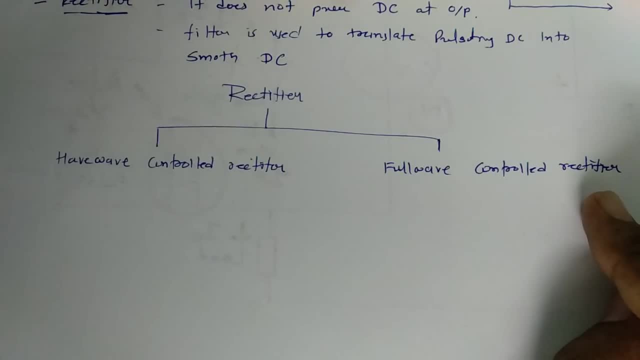 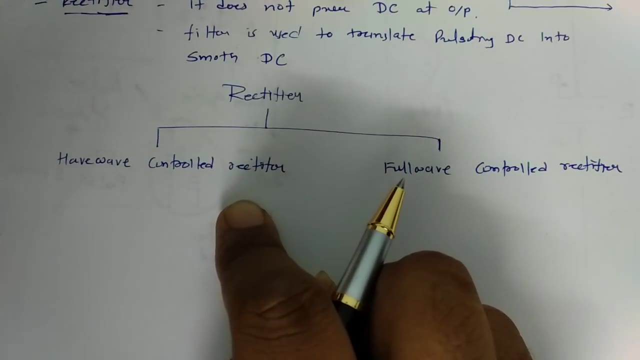 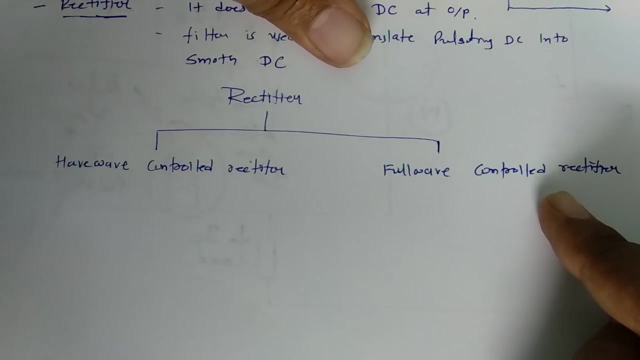 wave translation of input to output in terms of DC. so we'll be having full wave translation of input to output in terms of DC, while in case of half wave controlled rectifier we can have half wave translation into DC from AC. so even in full wave, I'll explain how many things that we can control and in full wave there are two. 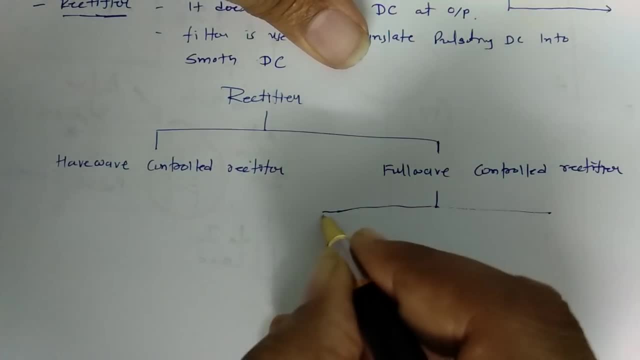 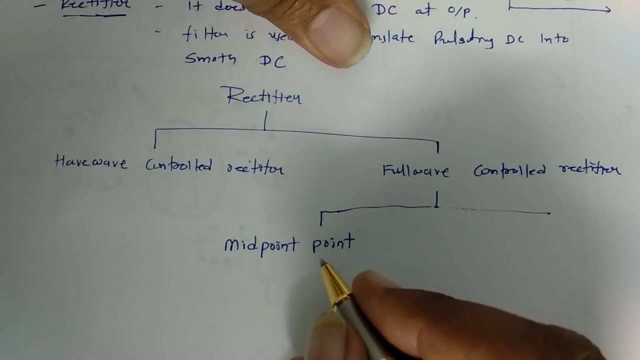 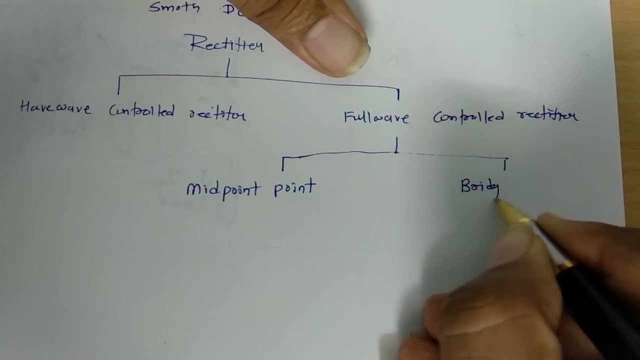 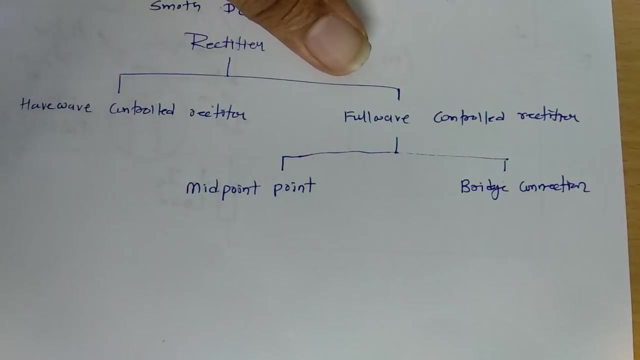 different types that I'll be explaining. first is midpoint connection, where we'll be having a transformer that will be center type transformer, and in second type I'll explain bridge connection. so in bridge connection we don't need to have center type transformer and in that, by connection of two types, we can have a center type transformer. 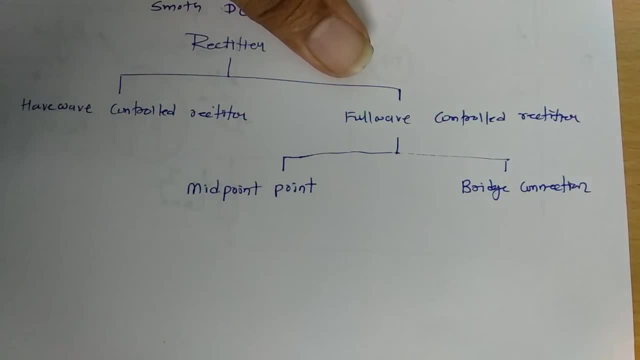 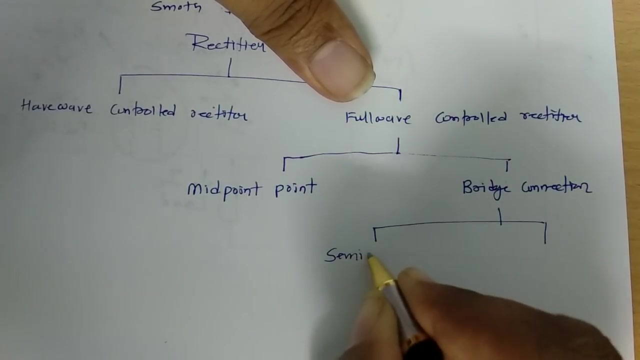 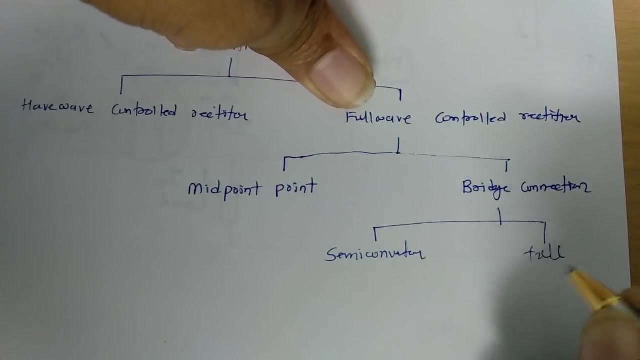 by connecting bridge configuration we can translate AC into DC. so this is what I'll be explaining in full wave controlled rectifier and in bridge connection I'll explain again two things. one is semi converter and second is full converter. so in semi converter for a bridge connection i'll explain how we can have a connection with. 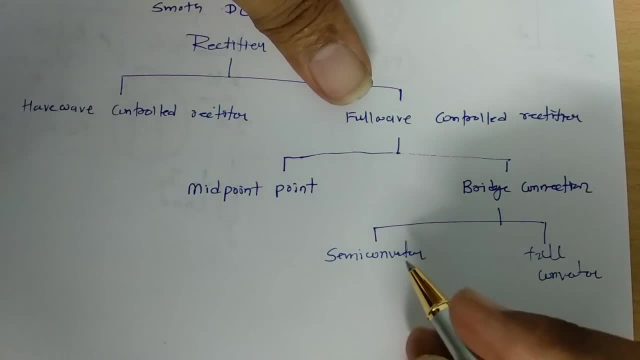 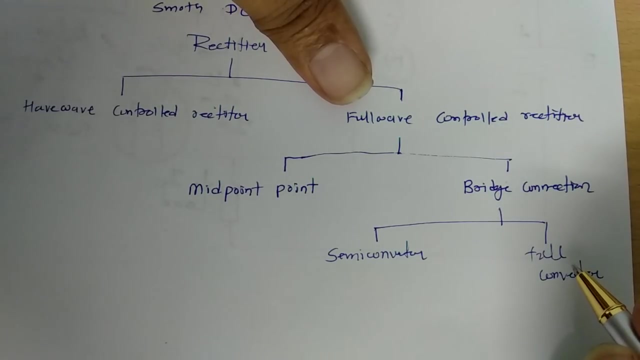 scr as well as diode. so in semiconductor we connect a bridge with two scr and two diodes, while in case of full converter we can connect four scrs which will be converting full wave ac into full wave dc. and this is what the basic thing which i'll be covering in my 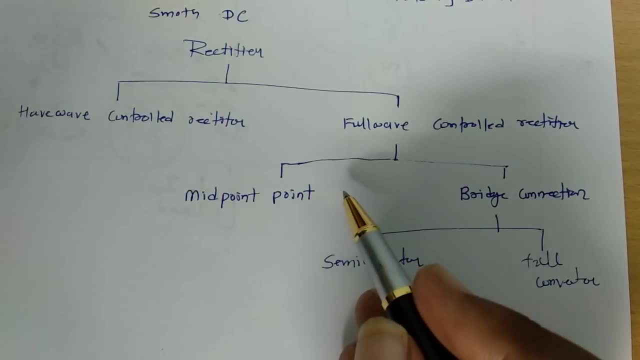 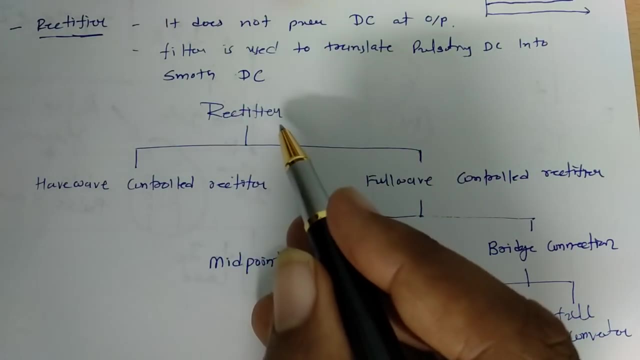 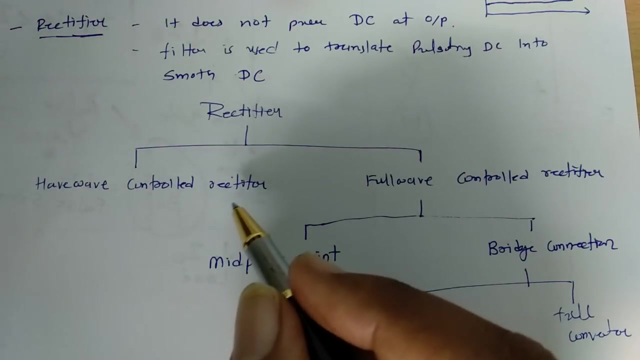 next sessions. and here i'm giving a brief idea about this now. here there is a difference in between rectifier and controlled rectifier. in rectifier circuit we can convert ac into dc, but in controlled rectifier we can control dc voltage, which is happening at output side. 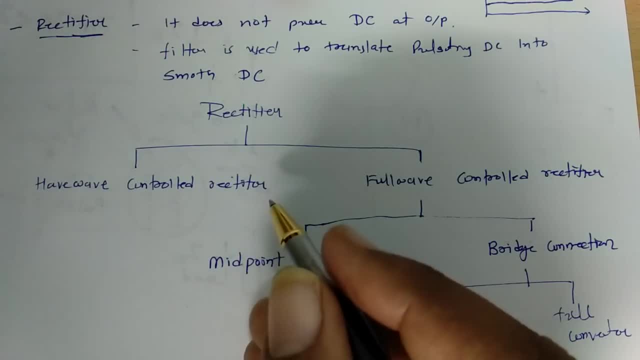 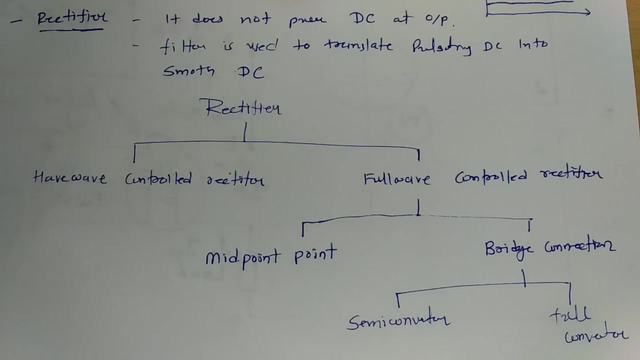 and that that is possible by connecting scrs. and in case of normal rectifier, we don't need to connect scr, we can make it by having diode connection. so that that is what the basic difference and what could be the triggering point, and all those things that we'll be discussing in my next sessions. so you 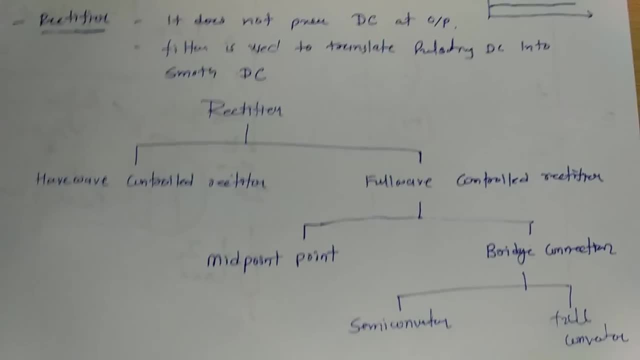 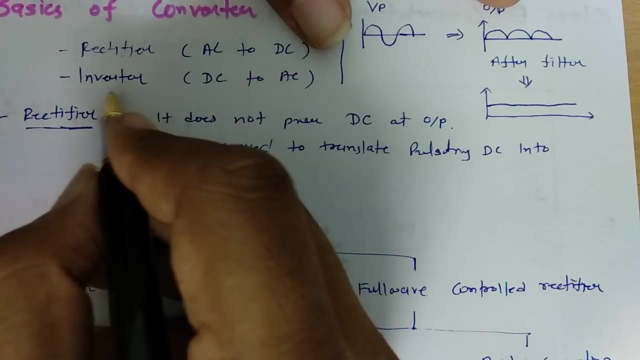 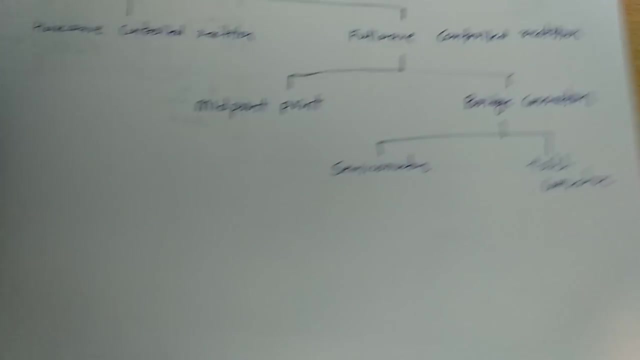 just stay tuned with my next sessions where i'll explain all those things. and second part, that, as i have earlier told, in converter it is including inverter, so inverter that translate dc into ac. so when you have dc input and you wanted to have ac output at that time, you need to have inverter. so inverter. 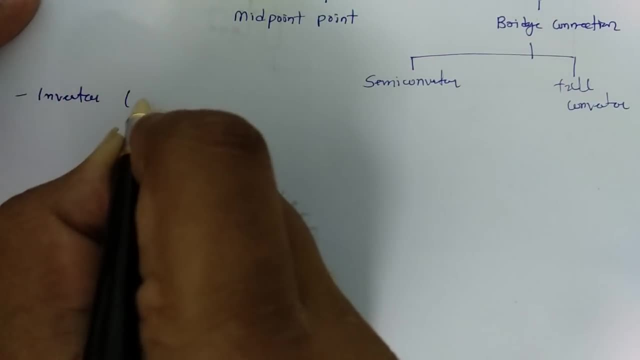 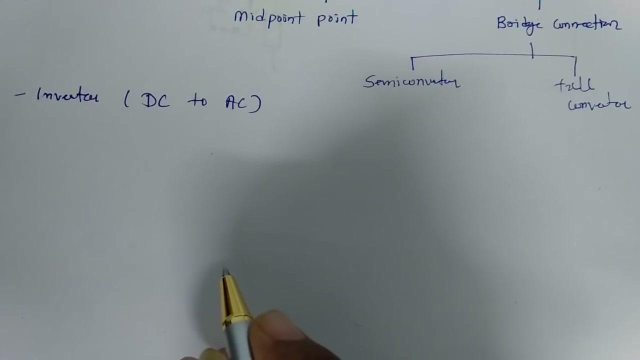 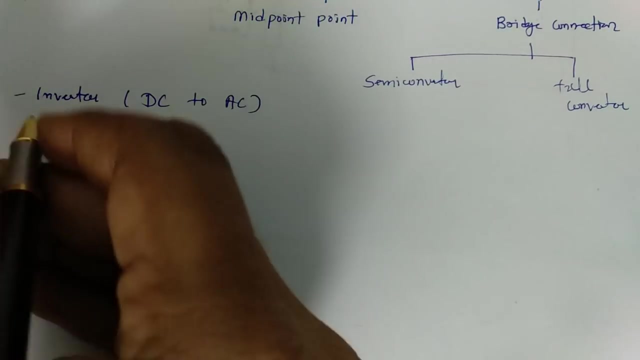 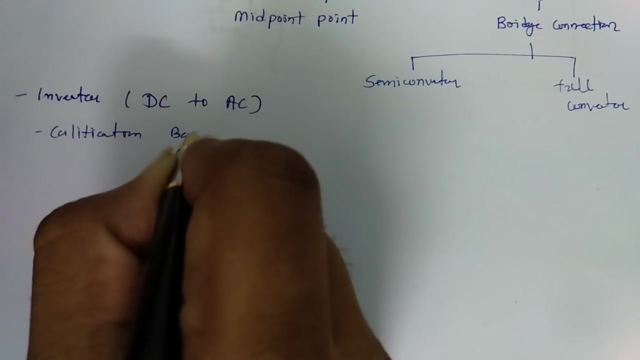 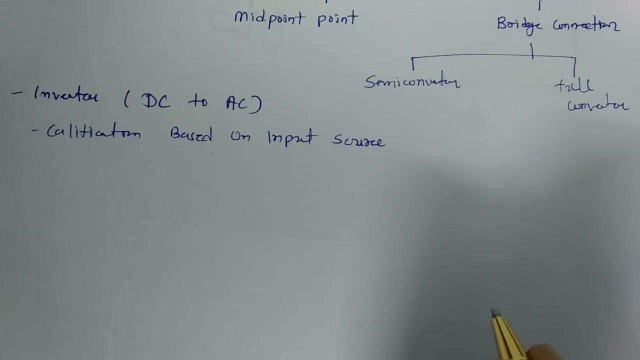 that translate dc to ac now based on its circuit connection. this is where you can have different types of classifications, where- first i'll explain- we can classify inverter based on input source. so classification based on input source, so classification based on input source. that could be vasi means. 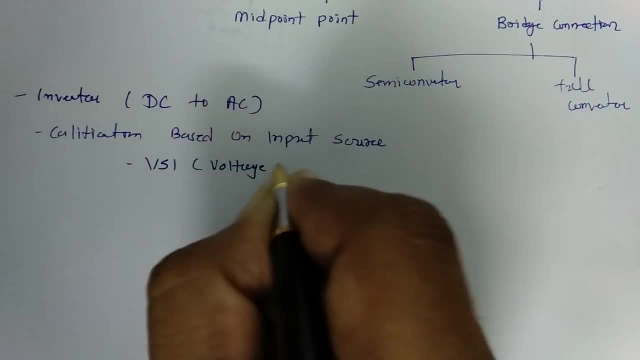 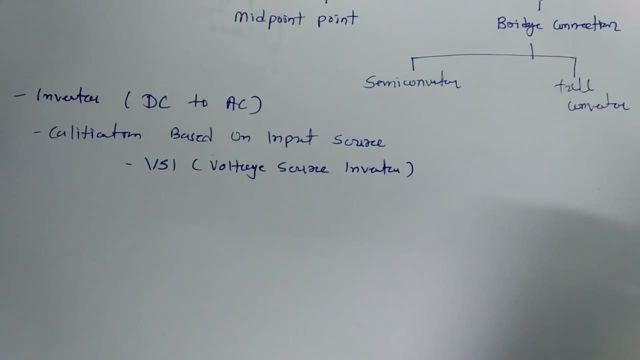 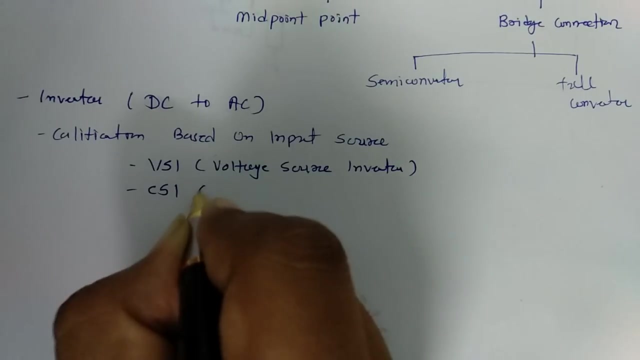 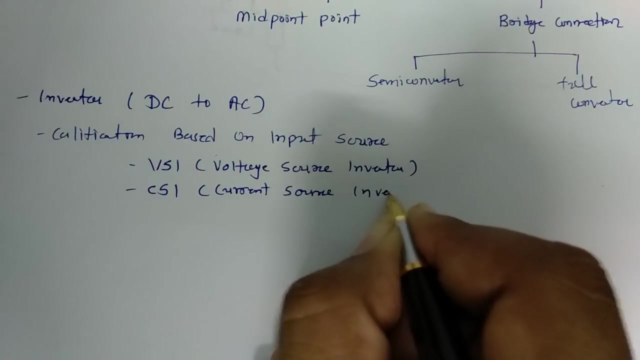 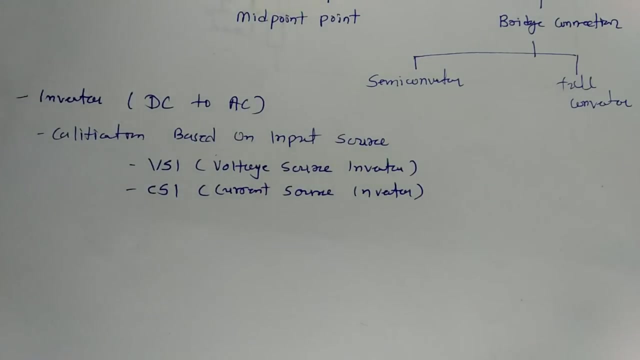 voltage source inverter. so if input source is voltage, in that case we can have voltage source inverter, where we can have DC to AC translation, and if input source is current source, in that case we can have CSI, where current source inverter could be utilized. so, based on input source, we can have two basic types: voltage source inverter and current. 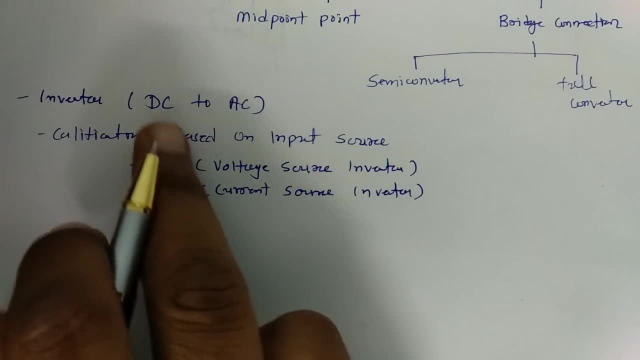 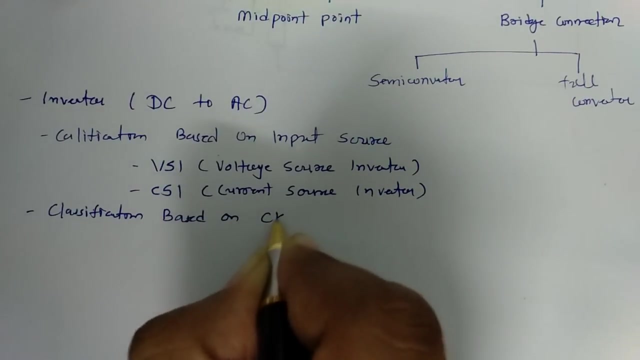 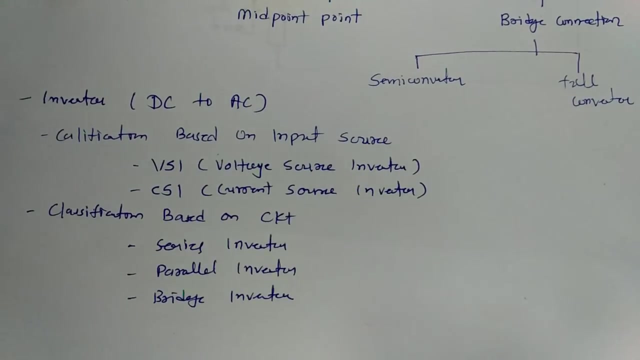 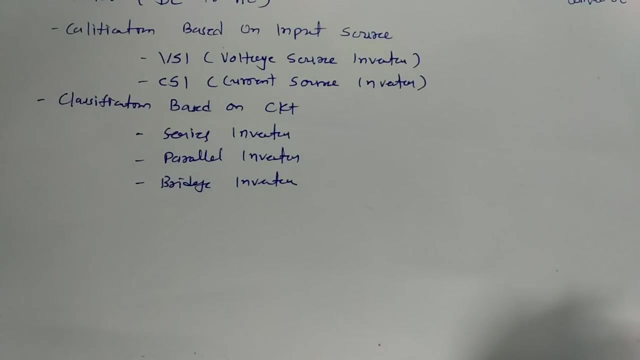 source inverter and functioning of that will be to have translation of DC into AC. now, based on circuit configuration, classification will be series inverter, parallel inverter and bridge inverter. so, based on circuit connection, we can have basic three types: series inverter, parallel inverter and bridge inverter. and based on type of output. 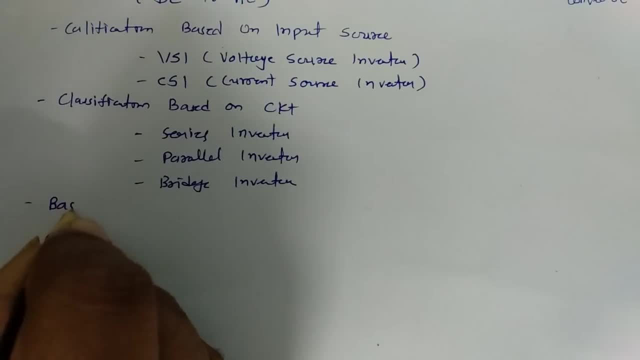 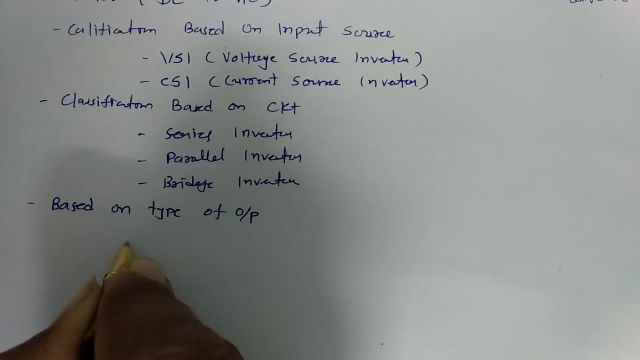 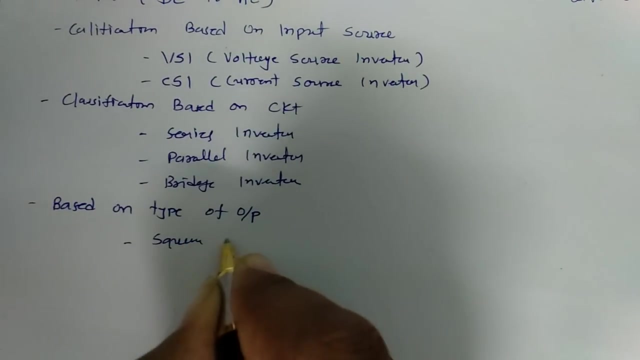 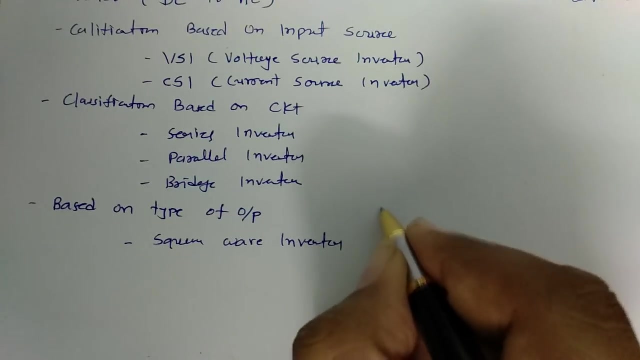 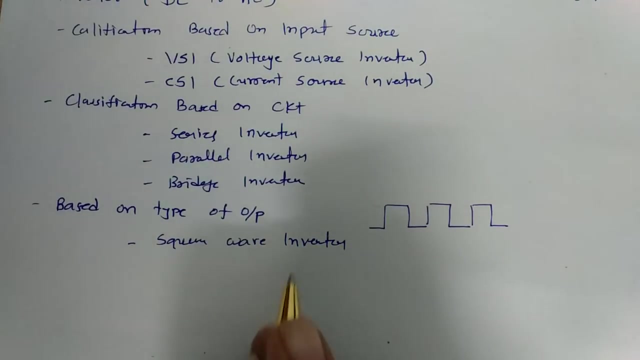 we can classify inverter. one is square wave wave inverter, where our output will be square wave, like this Say: if output is square wave, then there could be a type of inverter which is square wave inverter. there could be other type, like quasi square wave inverter. 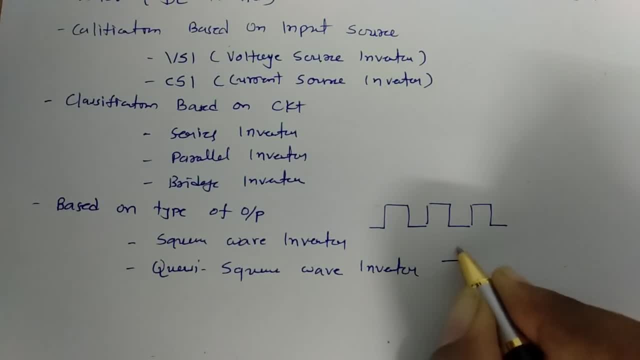 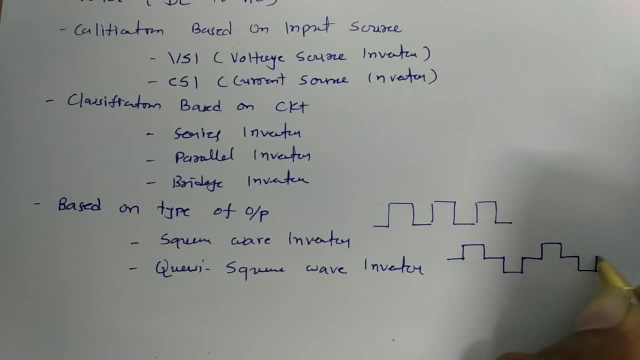 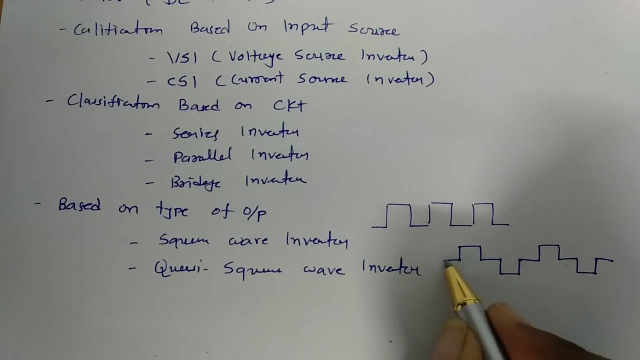 So in quasi square wave inverter our output will be somewhat like this. So quasi part- That is what we are translating into AC- and rest part will be zero. So here one can easily see: for this time interval output is zero and then positive half is there. 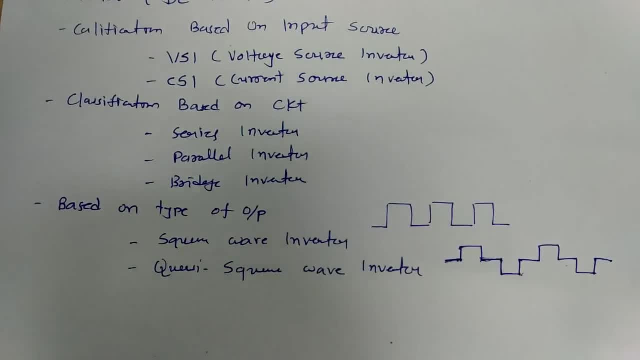 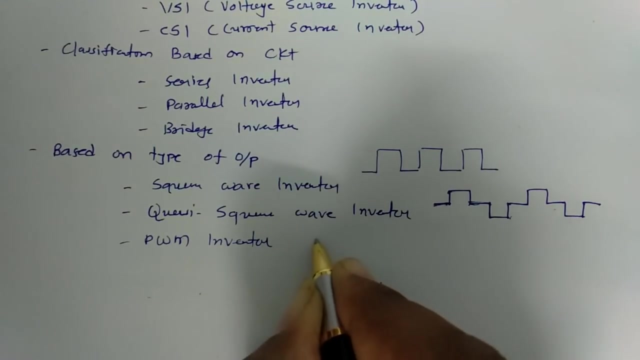 then again zero is there and then negative half is there. So this is what the output which is happening for quasi square wave inverter Next type, that is PWM inverter. So in PWM inverter we can have AC output and that is having pulse width modulated output. 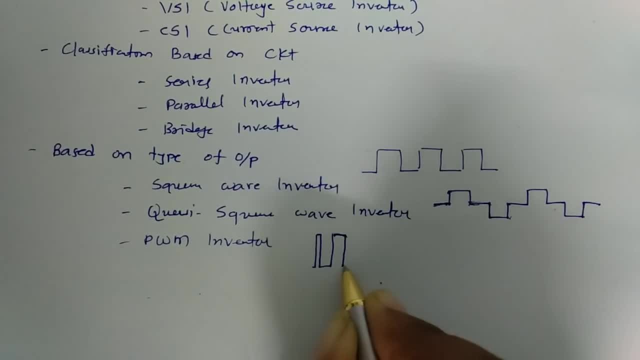 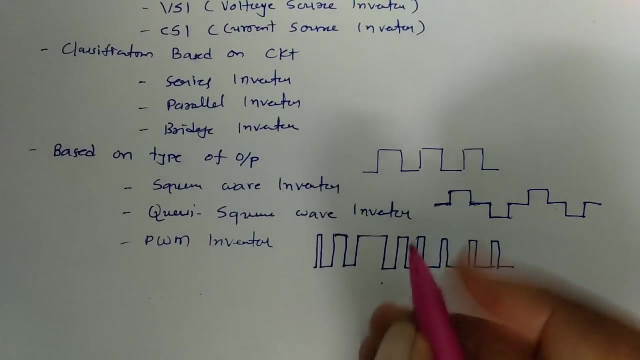 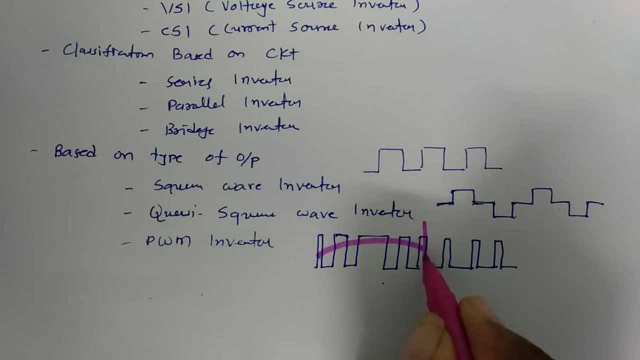 So one can try to understand how that happens, Like right now I am explaining this with this one output where one can clearly see So over here for this section. for first half section one can see average DC output is positive and for next half section one can see average DC output is negative.